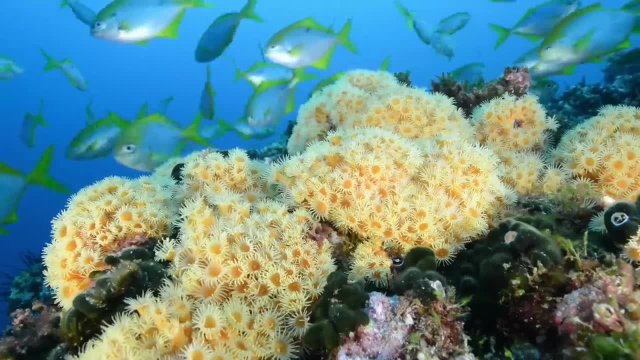 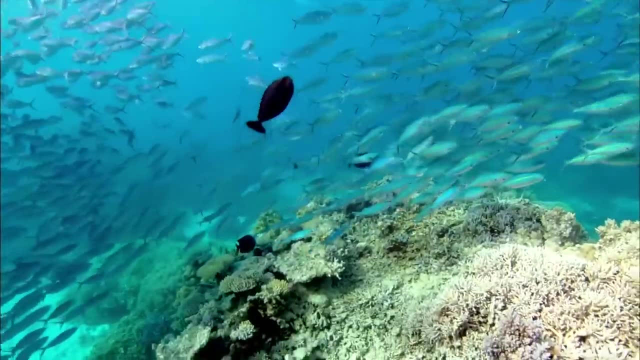 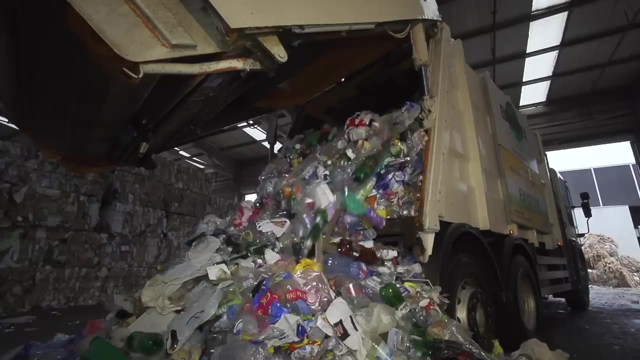 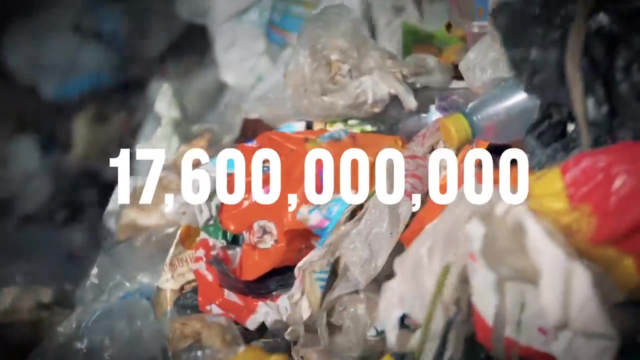 Our oceans sustain life. An abundant ocean can feed a billion people a healthy meal every day, forever. But now they are being filled, killed, by throwaway plastics. The equivalent of one garbage truck of plastic is dumped in the sea every minute. 17.6 billion pounds every year. 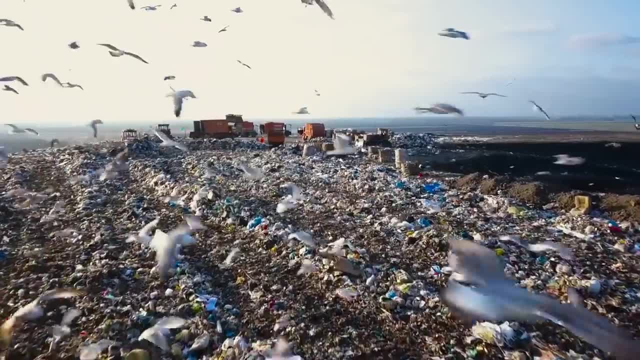 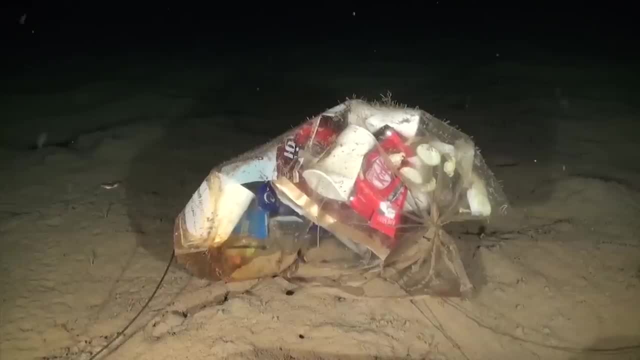 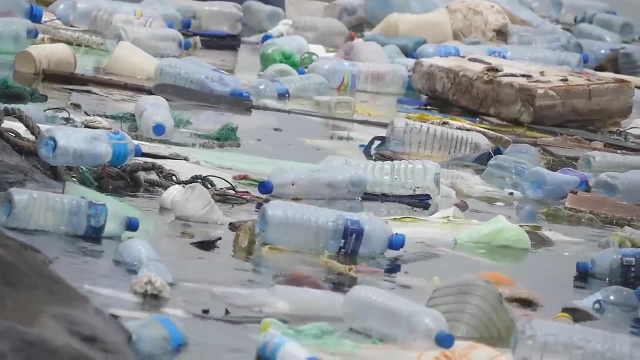 Plastic is everywhere in our ocean, Floating on the surface, mixing in the salt water and sitting on the ocean bottom miles and miles deep. And once in the ocean, it never goes away. Over hundreds of years it breaks down into small pieces. 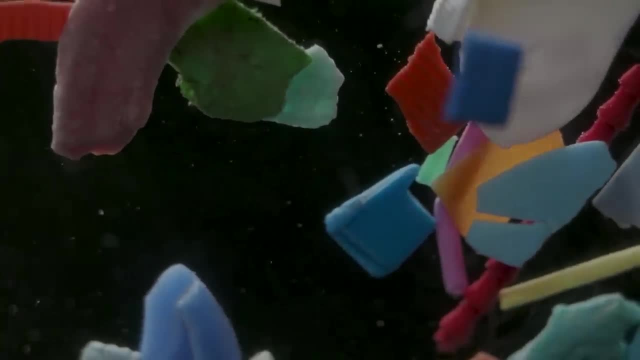 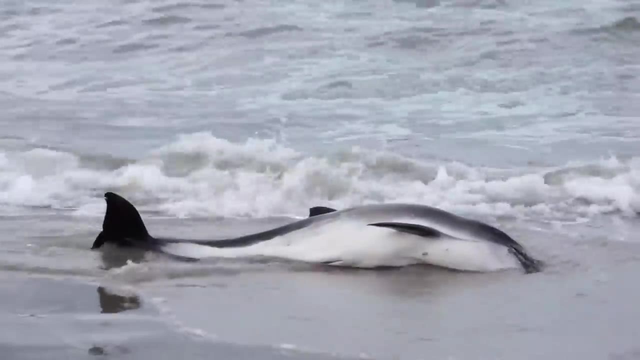 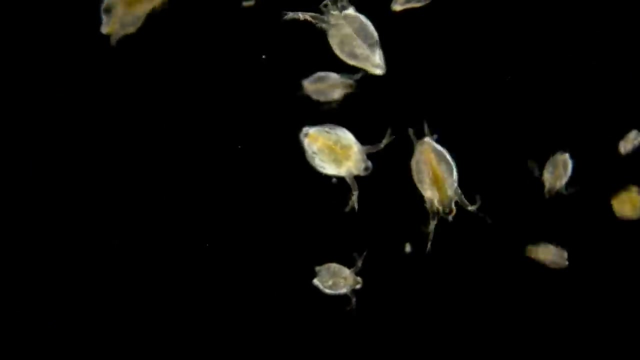 But those pieces, even the tiny ones called microplastics, are still plastic. Sea turtles are choking on it. Scientists say that over 60% of whale and dolphin species are affected by it. Zooplankton, the base of the ocean food chain, eat it. 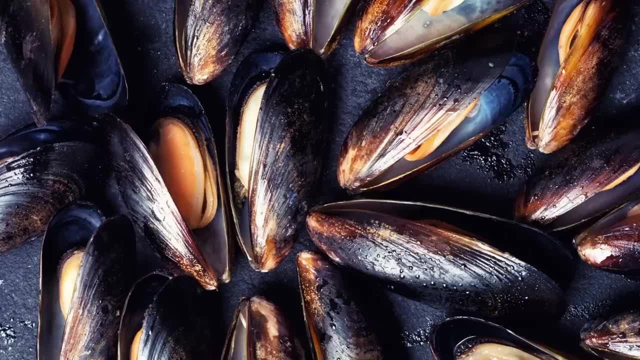 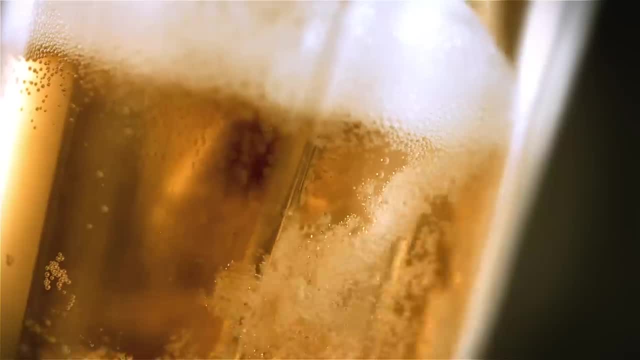 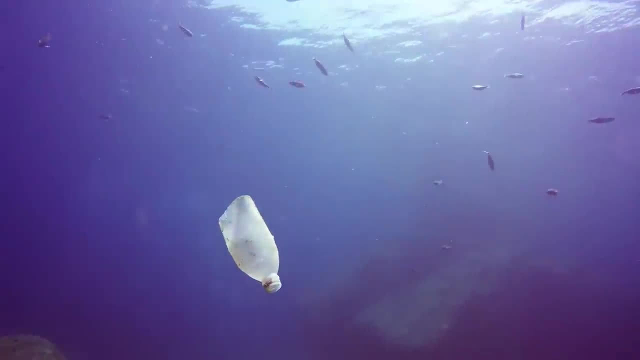 And so do we. It's in the water we drink, It's in our food. Microplastics have been found in our salt, our honey and our beer, And sometimes even in the air we breathe. Companies are choosing to make something. 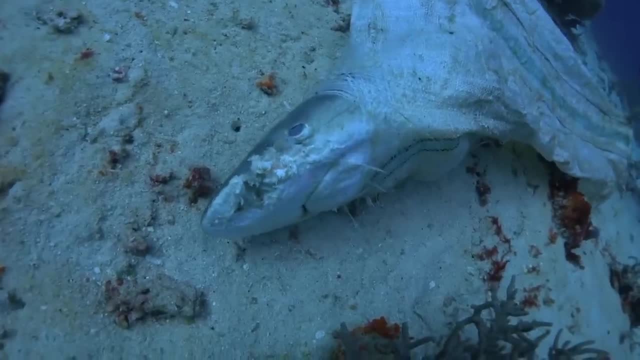 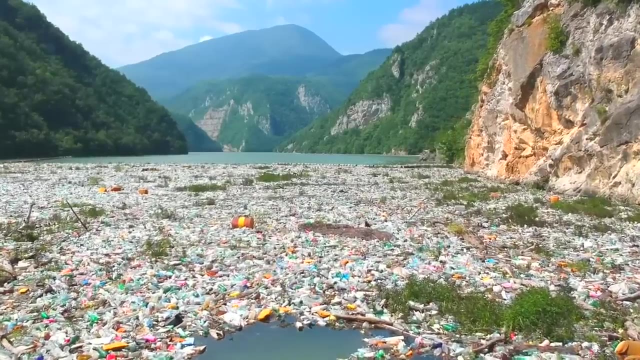 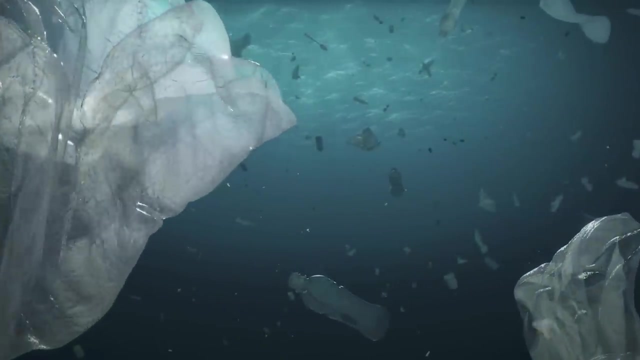 that will be used just once, from a material that lasts forever. If you don't like what throwaway plastics are already doing to our world, brace yourself. We face a tsunami of throwaway plastic in our and the ocean's future. Four times more plastic will be produced between now and the middle of the century. 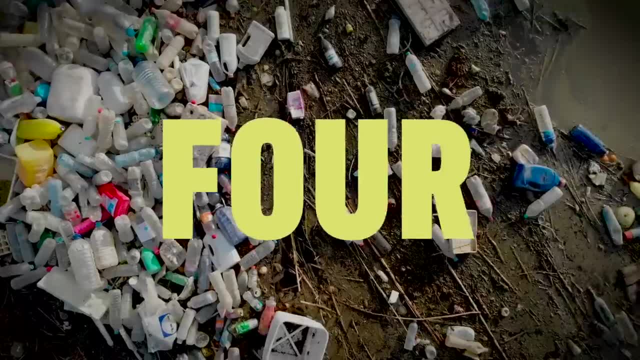 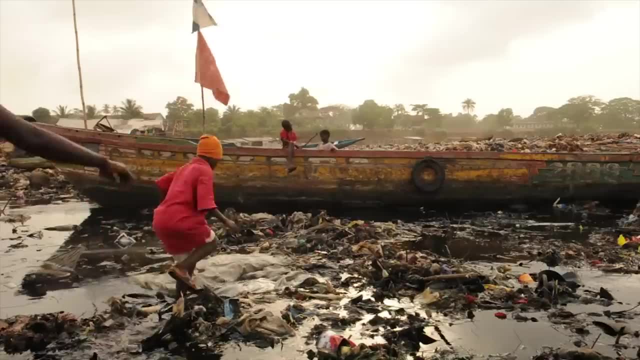 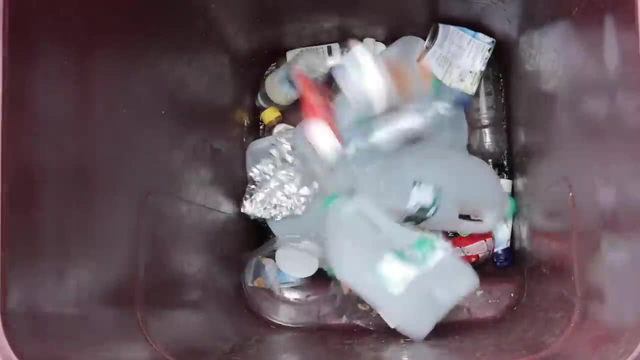 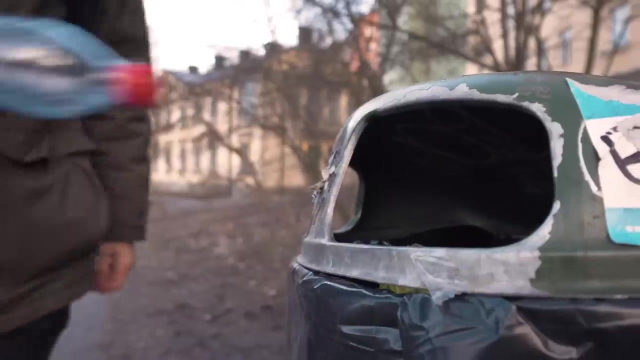 than has been produced in all of history- Four times more. What can we do? Recycling Of all the plastic ever generated as of 2015,. only 9% was recycled. Even when it is recycled, plastic degrades. Your plastic soda bottle maybe becomes a shampoo bottle, then a floor mat.